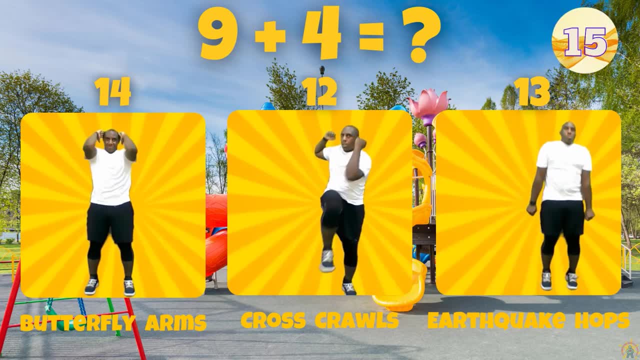 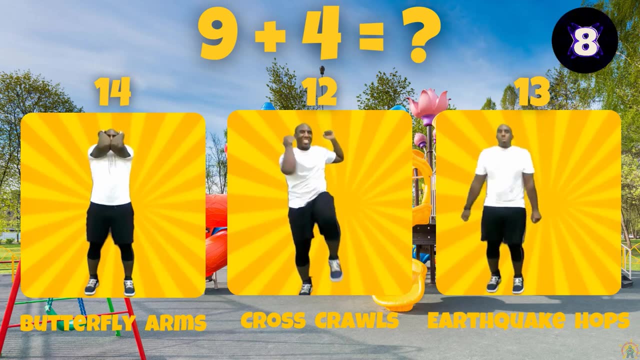 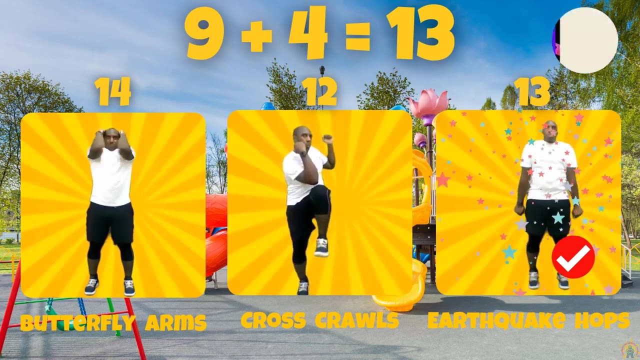 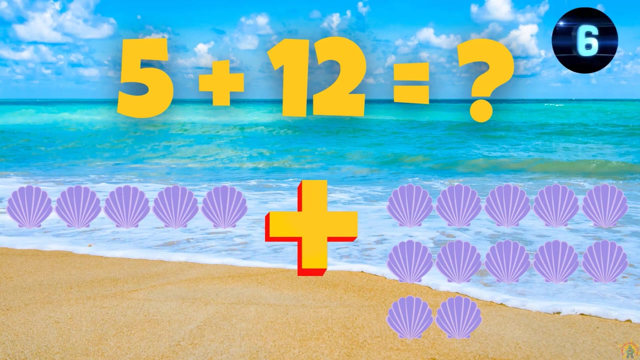 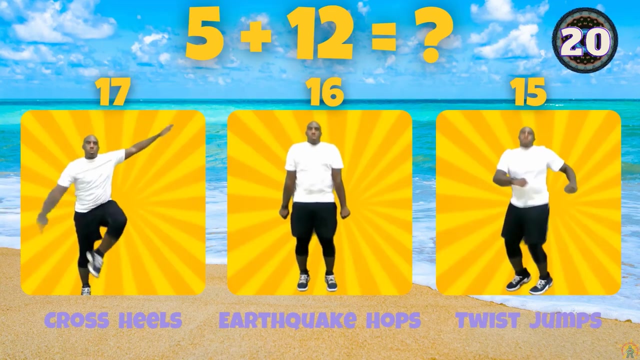 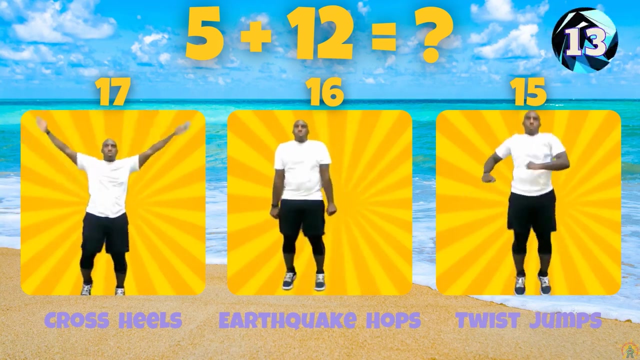 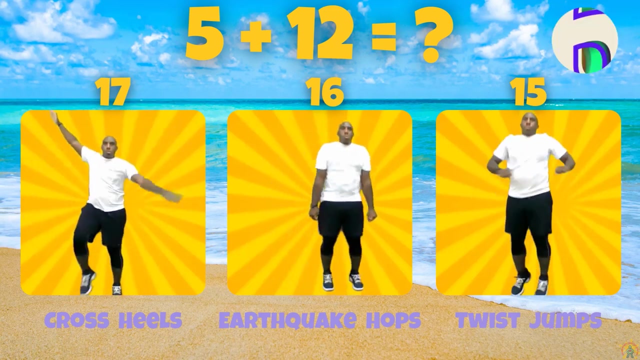 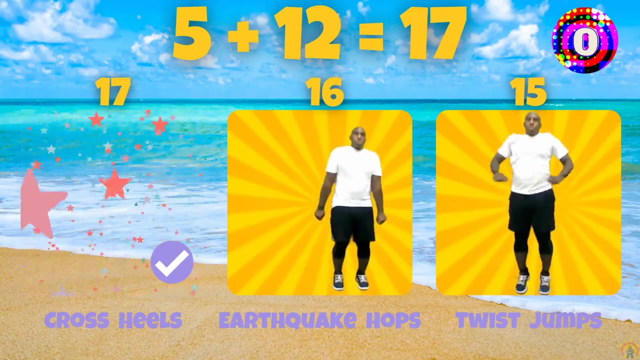 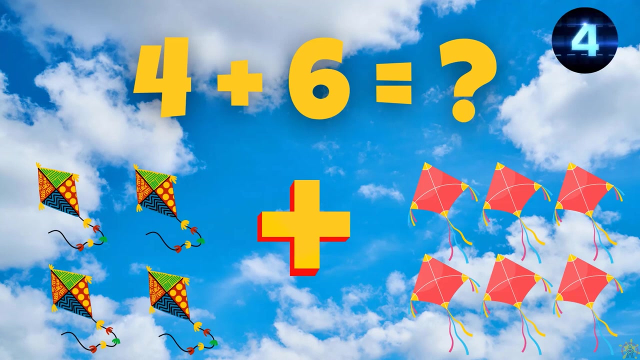 9 plus 4 equals- Is it 14,, 12, or 13?? That's right. nine plus four equals thirteen. Five plus twelve. Five plus twelve equals seventeen, sixteen or fifteen. Yes, Five plus twelve equals seventeen. Four plus six. 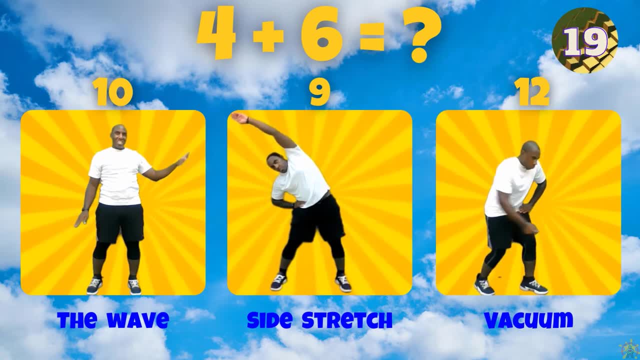 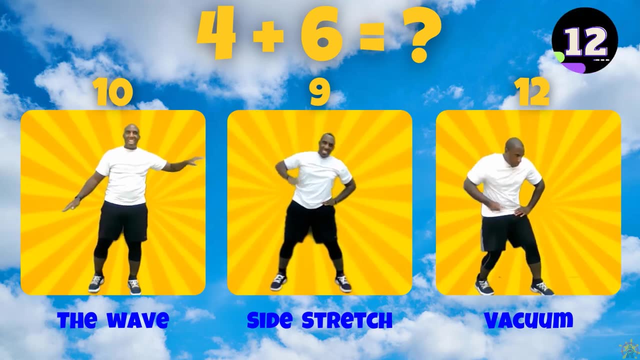 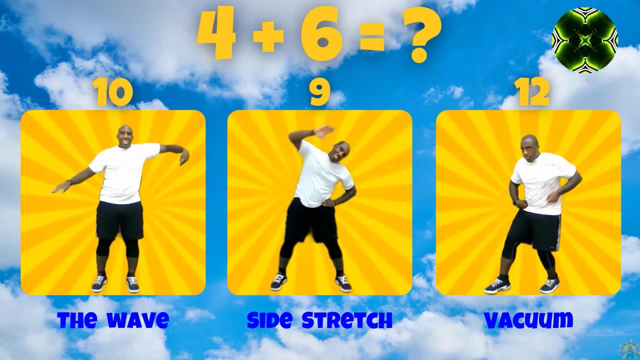 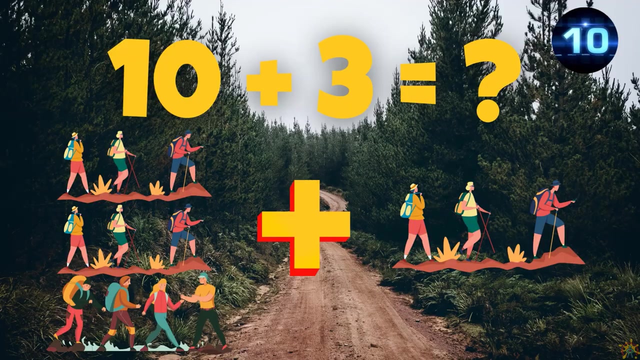 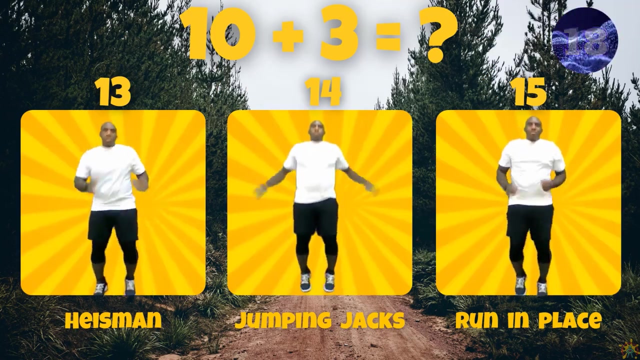 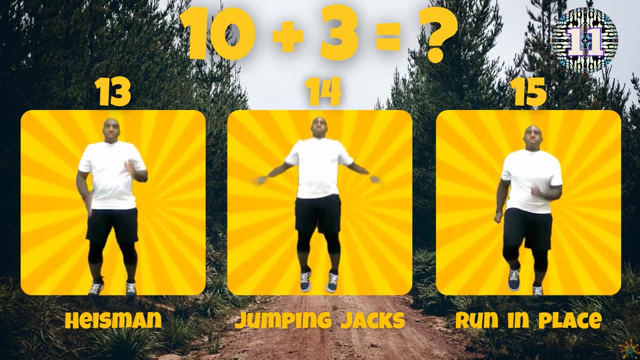 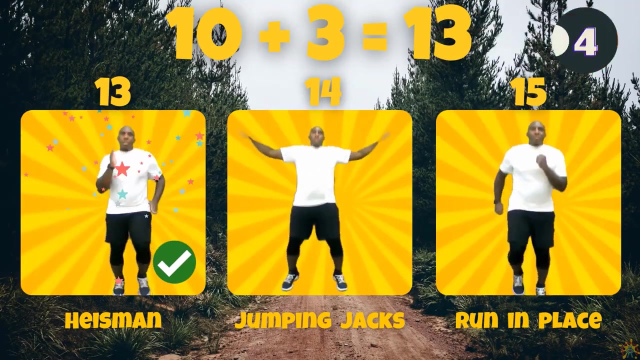 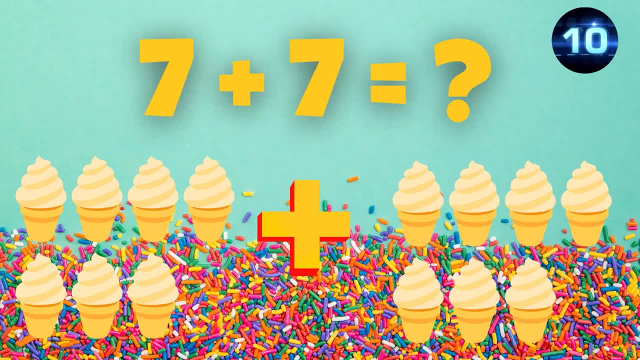 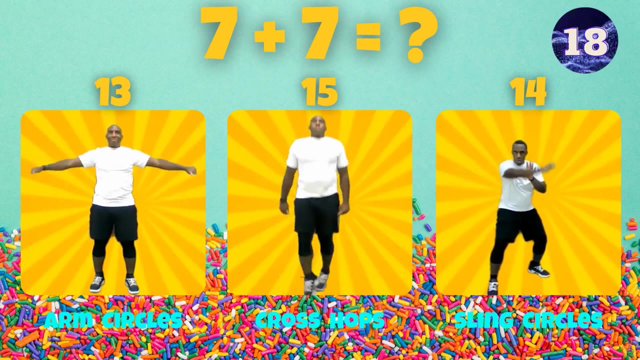 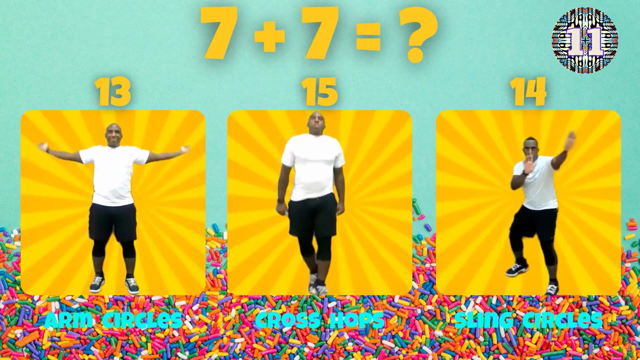 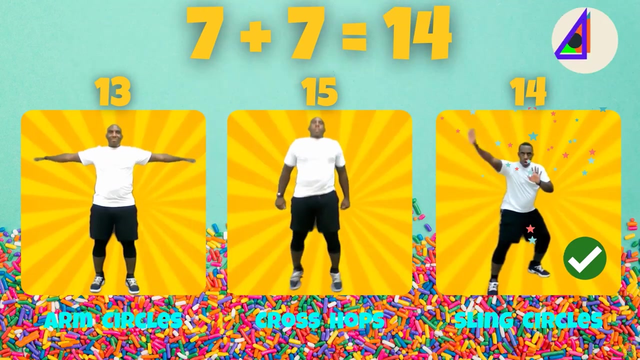 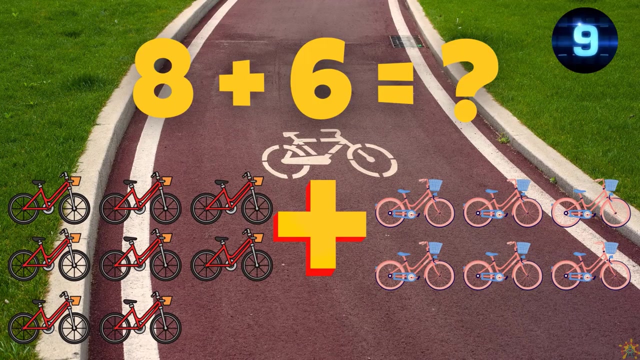 Ten plus three equals thirteen, Seven plus seven. Seven plus seven: does it equal thirteen fifteen or fourteen? Yes, Seven plus seven: does it equal thirteen, fifteen or fourteen? Yes, Oh yeah, Seven plus seven equals fourteen Eight plus six.